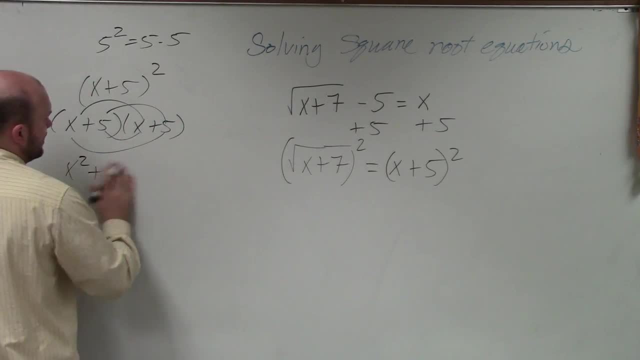 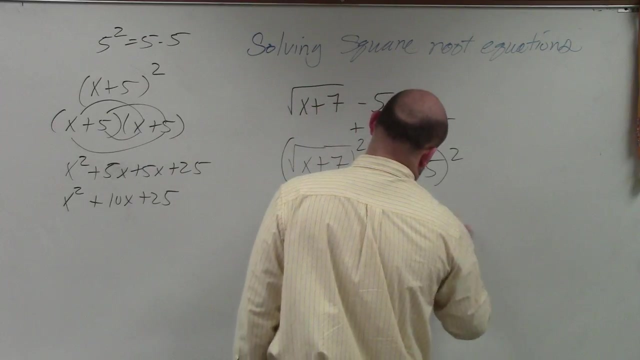 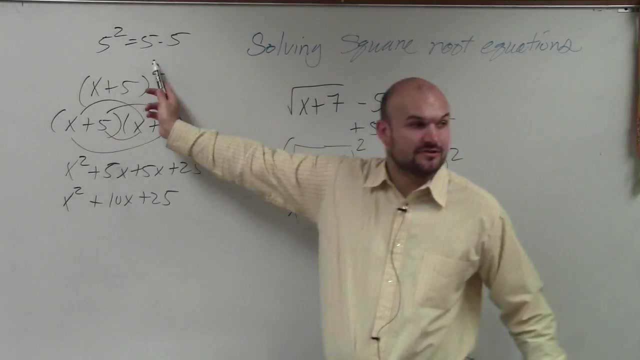 And what you'll see is that's x squared plus. I'll just write it out: 5x plus 5x plus 25, which is x squared plus 10x plus 25.. I just did FOIL: x plus 5 squared is x plus 5 times x plus 5.. x times x is x squared. 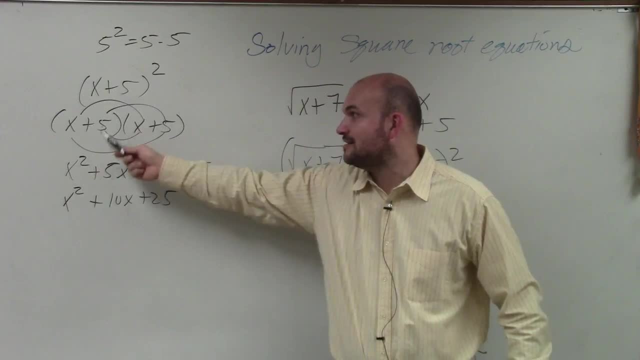 5 plus 5 squared is x plus 5 times x plus 5.. 5 times x is 5x. 5 times x is 5x. 5 times 5 is 25.. 5x plus 5x is 10x. 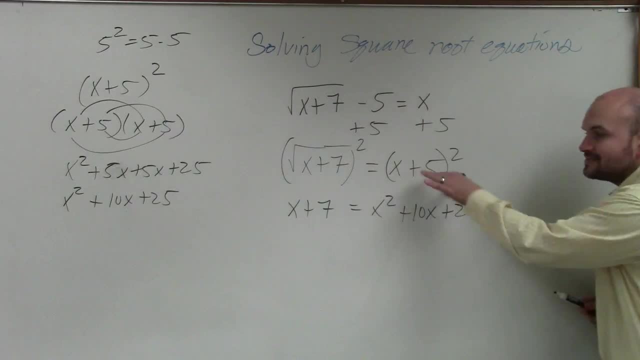 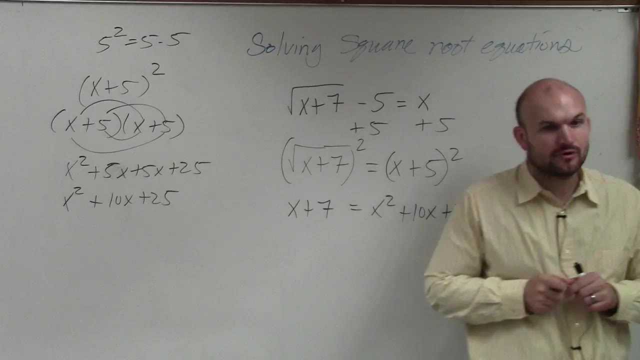 Have you seen that, Justin? Okay, So x plus 5 squared guys is a trinomial. Now you guys can see we have a quadratic. Oh, we talked about solving quadratics. We can't solve quadratics using linear properties. 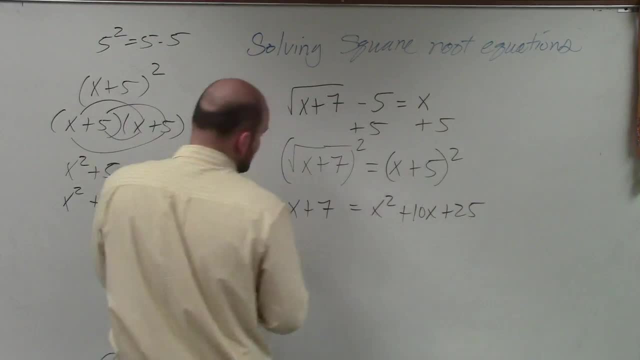 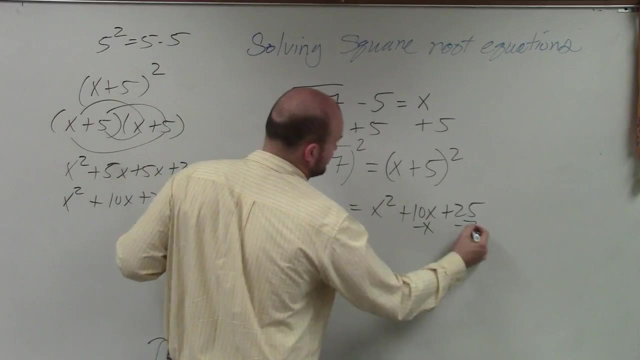 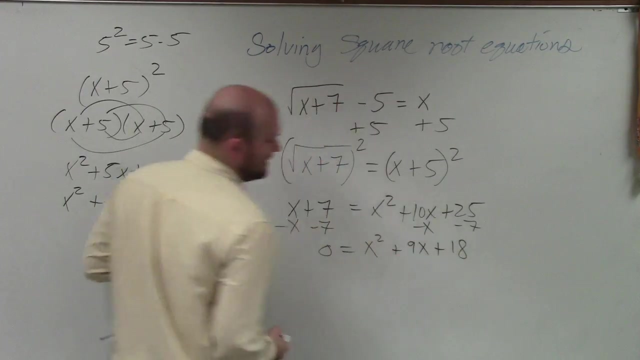 What we're going to have to do is use factoring, So I need to. to do factoring, though we have to set it equal to 0.. So I subtract an x And I subtract a 7.. I have 0 equals x squared plus 9x plus 18.. 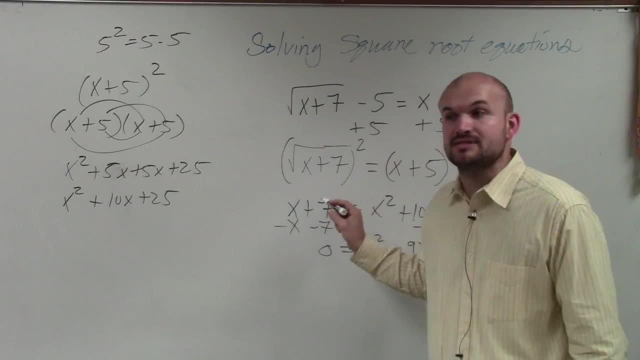 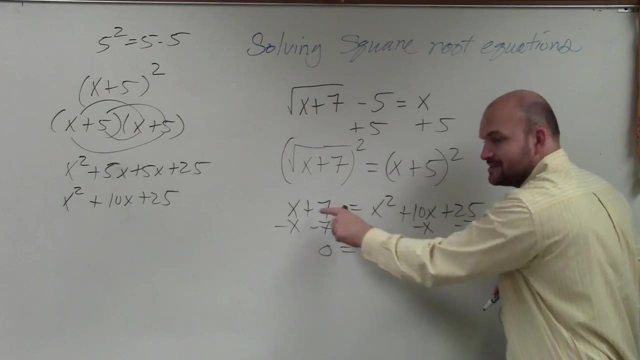 Oh man, But you have to get rid of these. You have to set them equal to 0.. So to undo adding x- I can still watch you- you subtract them on both sides. And then adding 7, you can subtract the 7 on both sides. 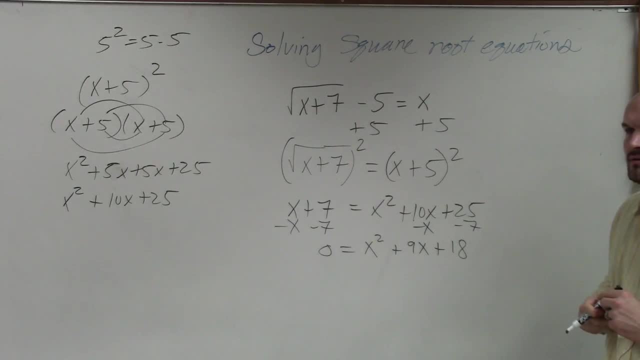 So now it's set equal to 0.. Okay, Okay, So now we need to factor this. Well, if you're going to go ahead and factor, ladies and gentlemen, remember we have 18 and positive 9.. What two numbers multiply to give? 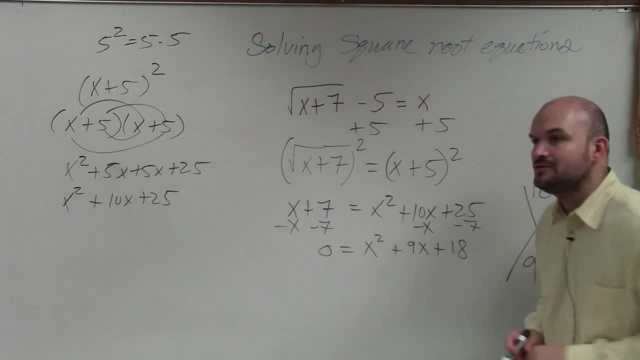 What two numbers? multiply to give you positive 18 and add to give you 9? 2 and 9.. No, What are all the two numbers? 1 and 9.. You're right, 2 and 9 do would give you multiply to 18.. 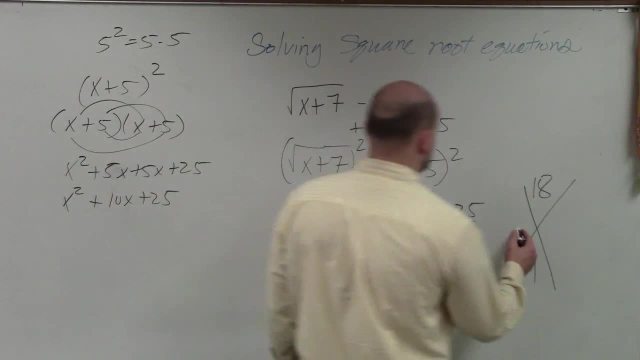 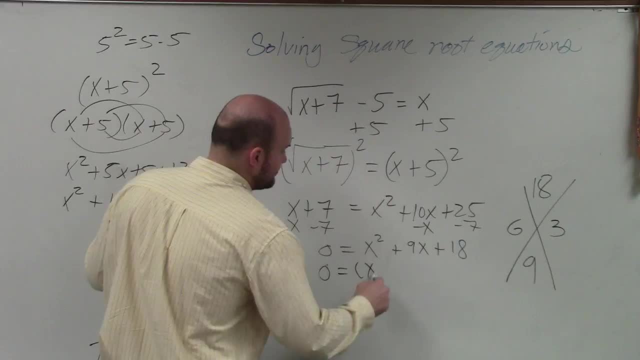 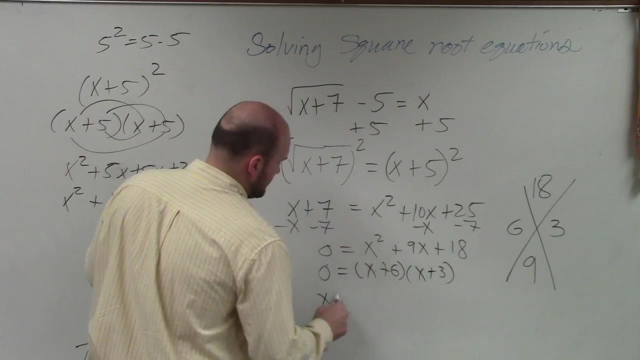 1 and 2.. 1 and 2.. 1 and 2.. 1 and 3.. So now x plus 6, x plus 3.. x plus 6 equals 0.. x plus 3 equals 0.. 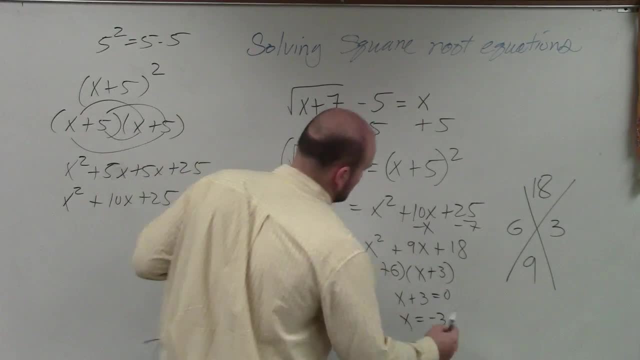 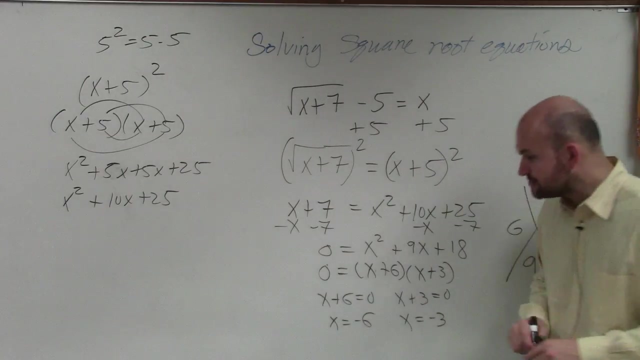 Okay, So now we have our two solutions, But, as I mentioned to you guys, the main important thing is we have to make sure we go back and check our answers. So if we go back And plug in our answers back into our equation, 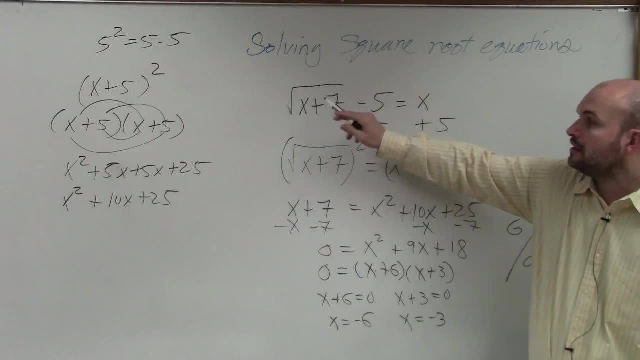 Let's plug in negative 6.. Negative 6 plus 7 is 1.. The square root of 1 is 1.. Right, 1 minus 5 is going to be negative 4.. And if I plug in a negative 6 for here, that's not going to work. 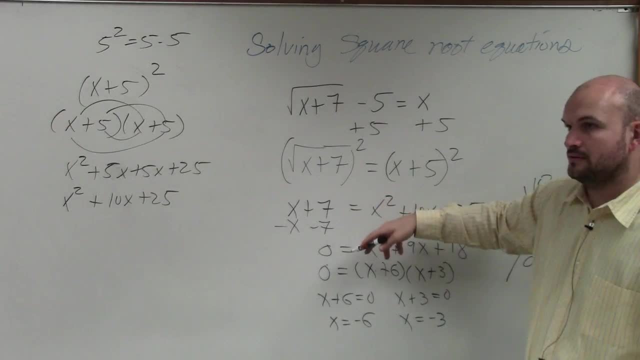 Do you guys agree with me? Yeah, I guess. yeah, Sure, No, Yeah, We're going to figure out a way of doing this. Sure, 1 minus 5 is negative 4.. Okay, Let's plug in negative 3.. 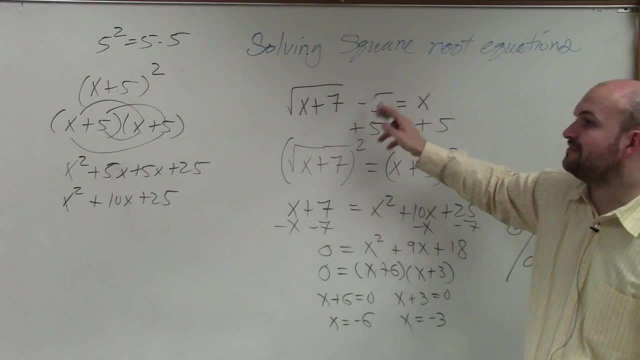 Negative. 3 plus 7 is 4.. The square root of 4 is 2.. 2 minus 5 is negative, 3. And if you plugged in negative 3 in for the sex, you would have negative. 3 equals negative.